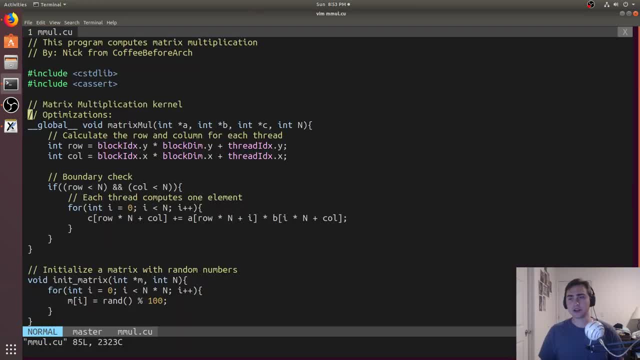 for arch. So the first thing we're going to look at is, you know, a very basic implementation. So here we've got, you know, matrix multiplication in global memory. So again, we're not using shared memory here. we calculate a row and a column right. this, with every single thread, is going to map to one output element in the C matrix, And then we accumulate inside of the C matrix. you know all these temporary results, And so by the time this for loop completes, we've got our final result in our 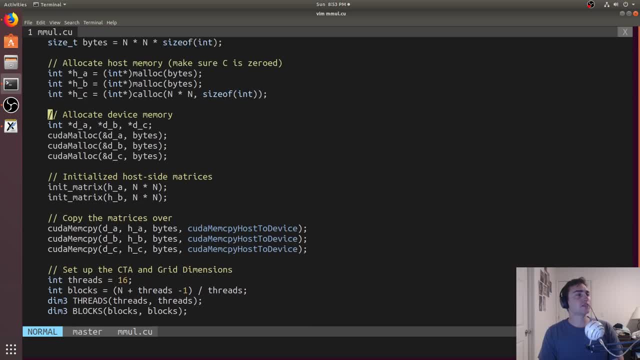 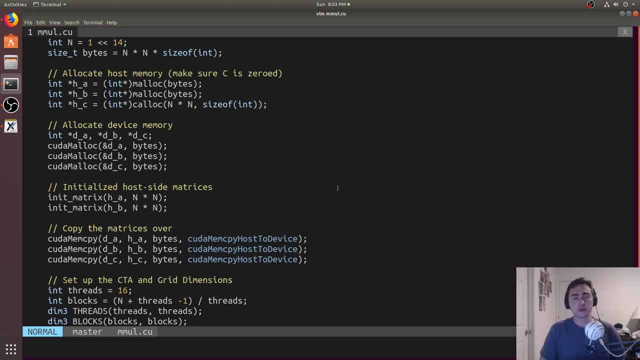 C matrix. So what has the main function look? a lot of basic things. So you see, we're not going to be using unified memory here because we really want to isolate the performance here. We don't want. you know, maybe sometimes we get lucky in terms of page faults. we don't want any of those errors. we really just want to see what the performance is of the kernel in isolation. So here we've got C alloc here. this is just to make sure that our C matrix is initialized to all zeros, Right. and you see that we're using 16 by 16 thread blocks, So 256 threads per thread. 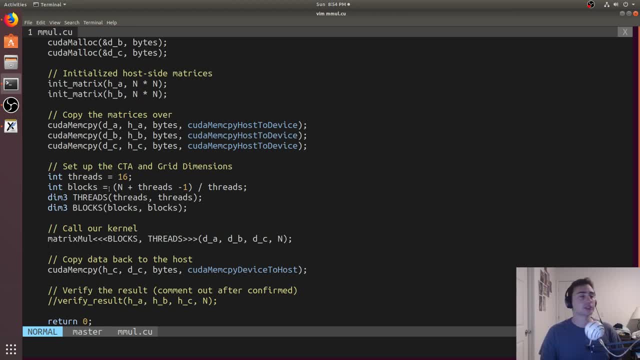 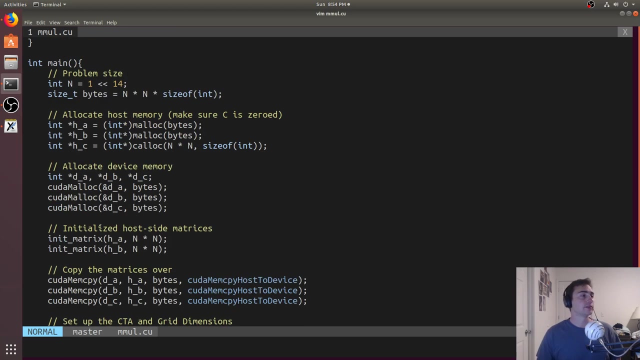 block 16 in the x direction, 16 in the y direction. And then, here you see, we pad out the number of blocks we need in both dimensions. So we launch blocks, comma blocks, right? So this dim three is just a struct with three fields, and x, y and z, And then we launch our kernel And we don't need to verify the results every time. So I verified the functional correctness of this. That way I don't have to verify it on these really large matrices. So all these performance results are for a 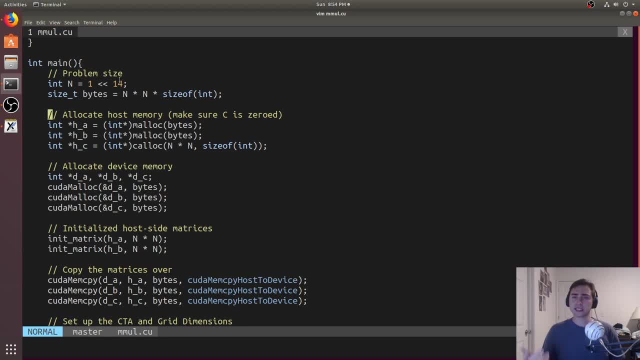 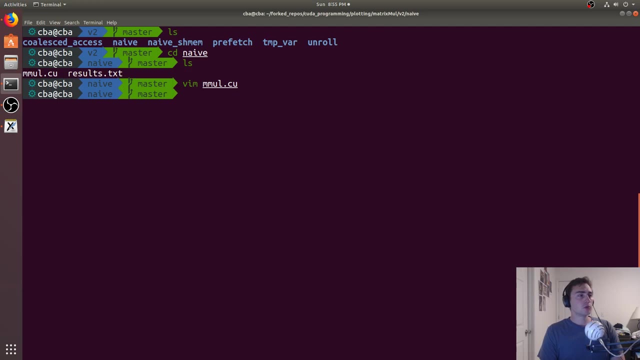 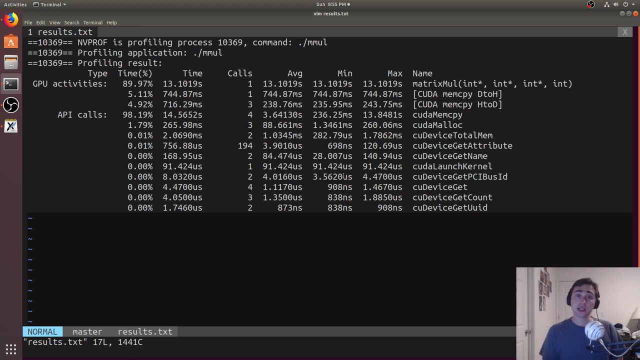 4096, or rather a two to the 14 by two to the 14 matrix, Right? so this is pretty big. each matrix is going to be gigabyte in size, right? so a gigabyte for a, gigabyte for B and a gigabyte for C, Right? so pretty, pretty long computation here. So, with this basic version, what is our baseline? So in resultstxt? so this is run on a GV, yeah, a GV 100 GPU, So it's a Volta architecture, pretty big machine, or big GPU. 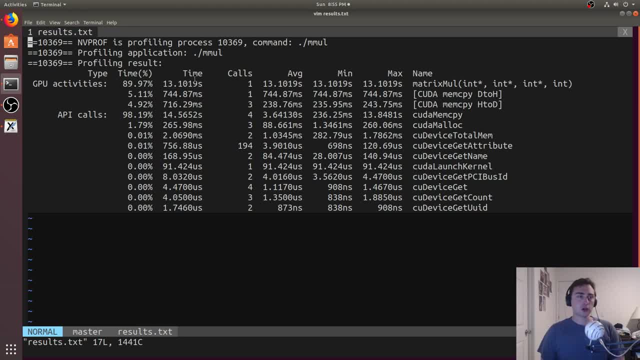 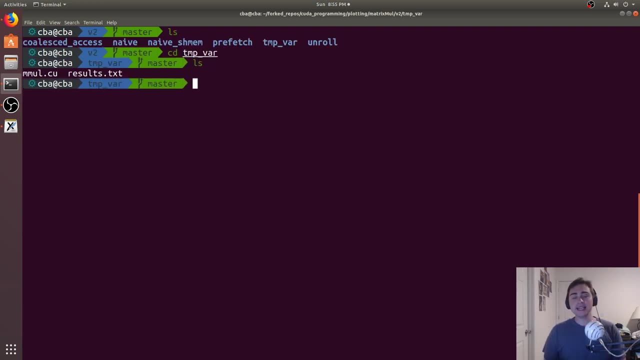 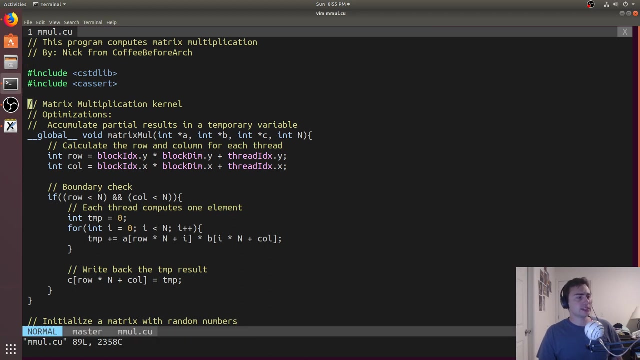 Right, and we get about 13 seconds right. So we don't really have any context. Is this good, Is this bad? But our baseline is going to be 13 seconds. So what's an easy optimization we can do? Now, the first thing we can look at is how do we maybe get rid of some unnecessary rights to memory? So let's open up this temp for one, And you see, the only difference that we do here is that, instead of writing back to memory every single time into C, we go ahead and use the 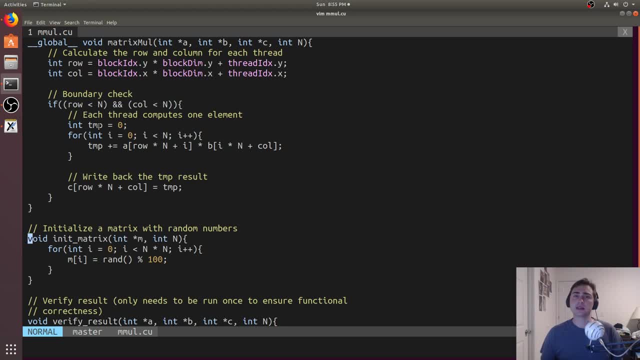 temporary variable. Pretty simple idea. Now what's the thought behind this? Well, if we can have temp and say a register, that means all we're doing is updating a register each iteration of this loop. That means we're not having to access memory. hopefully we hit on it in the L1 cache, maybe we don't, maybe we even miss in the L2 cache, And this way we can just avoid that altogether: have it in a register and then eventually have one write back. So we basically took you know in rights. 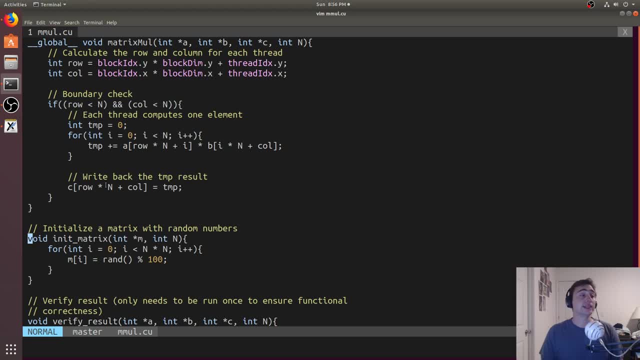 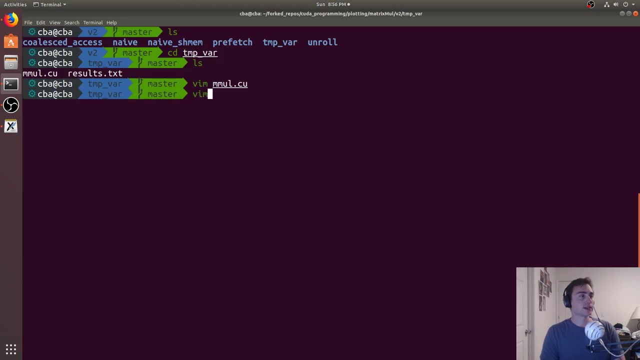 into memory with just a single write per thread. And you have to remember if we're launching, you know, you know, two to the 14 by two to the 14 threads, that means we're going to have two to the 14 times two to the 14 times two to the 14 rights to memory, right? Because we've got each of those threads we'll all be doing in iterations of this loop, Right? So we save all that. What does that give us in terms of performance? Well, here's our results, right from one run, And you see we're down from like 13 seconds to 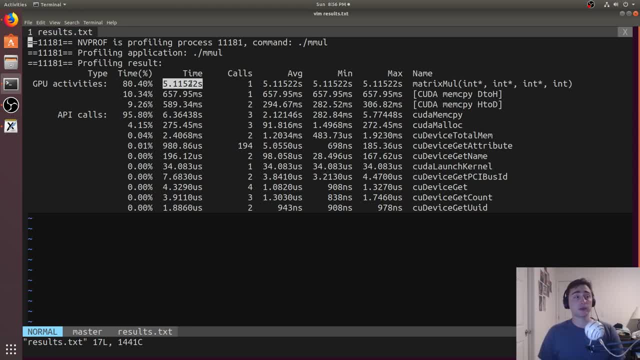 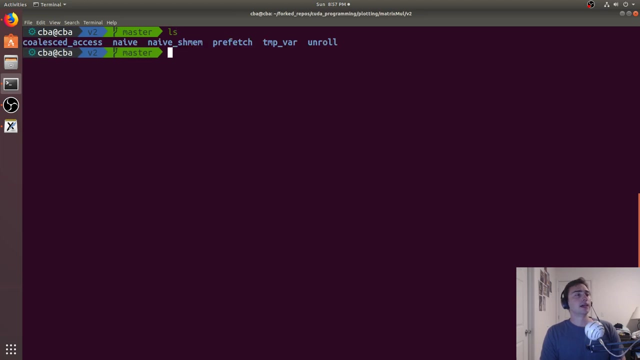 all the way down to five seconds, So that's pretty good, right? So we've already improved this quite a lot with you know. just about two or so lines of code, Right? So already we're seeing some basic optimizations here in terms of just eliminating some unnecessary work, But we can do even better than that. Again, this is all without shared memory, So what else can we do? Well, one thing that we didn't really talk about was our grid size, right? So grid size is a very 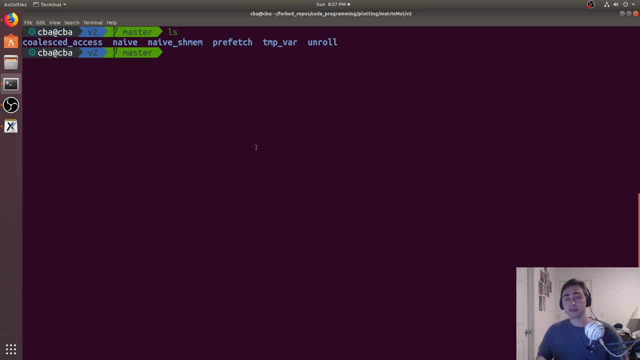 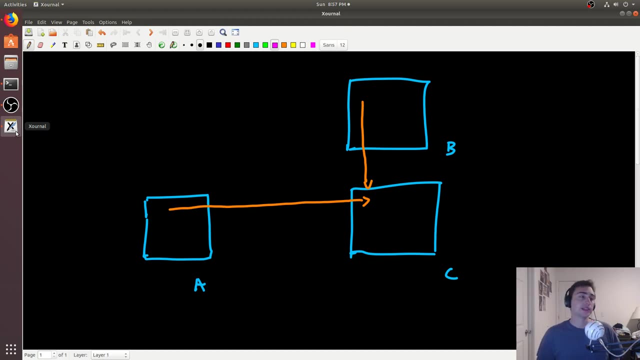 very important thing in GPUs and how we kind of lay out our problem and how that translates to performance. So let's go ahead and we'll kind of switch over. So this is basically what matrix multiplication looks like: We've got an A matrix, we've got a B matrix and then we have our C matrix, And every single thread will end up following this pattern of these orange lines. So it will go across the rows of this matrix, of the A matrix, and down the column of a B matrix, right. And so if we just added more orange lines, that would correspond to: 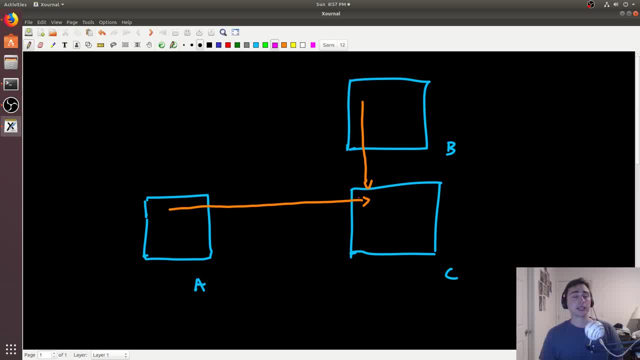 different elements of matrix multiplication. right, So each thread gets mapped to the C. So we'd have one thread here would follow this exact pair, right, So this row and this column. Okay, So what's a problem with our current implementation? So, right now, right, if we go ahead and consider that we have, you know, one thread block here, right, so that's going to correspond to just a chunk of our final matrix C, that thread block itself. so if we kind of expand this out, 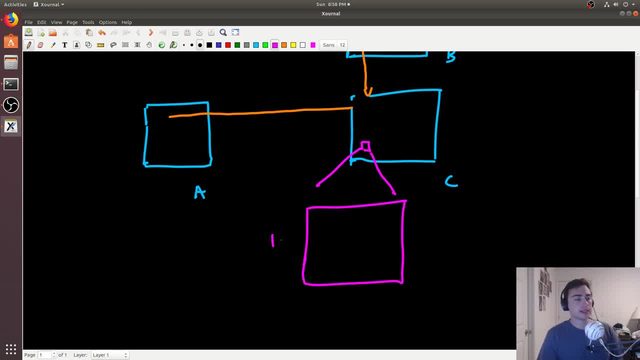 you know, we'll have, you know, 16 threads in this dimension. 16 threads in this dimension, right? So we go 16, blah, blah, blah, 16. And then we'll have you know more in that dimension. And let's go ahead and use a different color for this next row, maybe orange, right, And then a couple dots, right. So now we've got these purple threads right, So from zero to 15.. And then we have the orange threads, from zero to 15.. Now 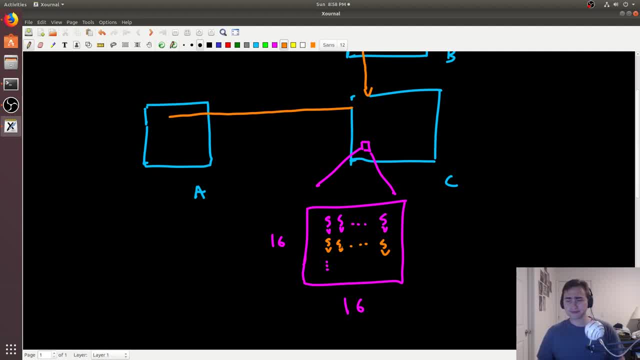 it's important to know that the SIMD width, or the width of the hardware, is actually 32, right? So you may have heard about warps, right, And warps are collections of 32 threads that execute together. So what happens? even if you have a 2d thread block or a 3d thread block inside of hardware, it has to get translated to. it has to be translated to a one dimensional thing, right? So all that thread ID x, thread ID y, thread ID z, those just correspond to values loaded from some special registers, right, For you know. 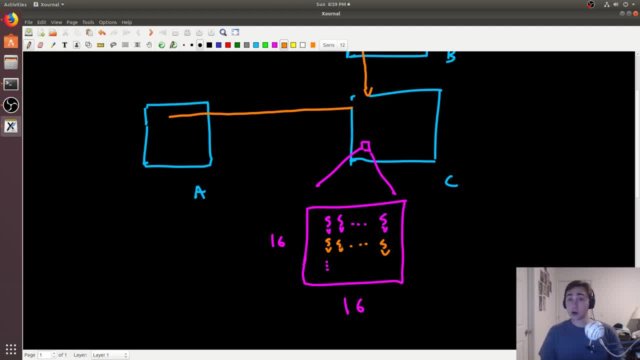 TIDs, right sort of thread IDs. So inside of the hardware, you know, it'll take some 2d arrangement like this of threads and it will go ahead and linearize it. And so how does that look? Well, here we've got 16 threads in the first row, 16 threads in the next row. So if it wants to make a warp of 32 threads, all it does is it pieces them together. So we'll have, you know, we'll have the 16 threads from this row And they'll get shoved together with the next row, right? So the 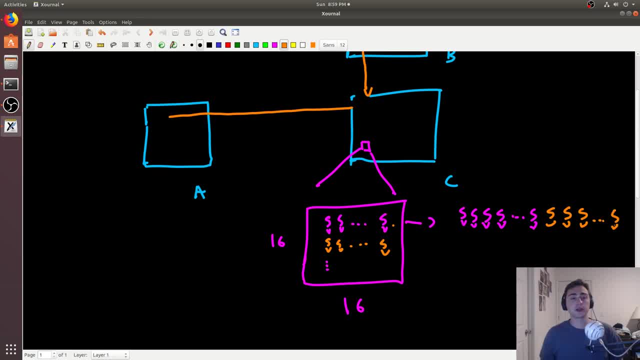 16 threads from the next row. So what's wrong with this? There's nothing inherently wrong with this. So if we think in terms of if we think in terms of things like control flow divergence, if, say, the purple threads went one direction and the orange threads went another direction, in terms of if we hit if statement, some go in the, if some don't, what ended up happening is only 16 of the threads maybe would be active at, you know, any given moment. So, effectively, those two 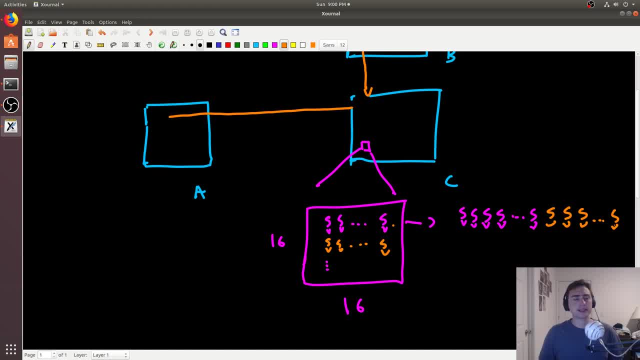 control flow paths get serialized right. So we don't have that in this case, because all the threads are going the exact same control flow path. So no control flow divergence. but we do have is memory divergence, though. So what ends up happening is these 16 threads will be accessing, you know, row zero, And these 16 threads will be accessing row one, And this is going to happen for every single warp, because every single 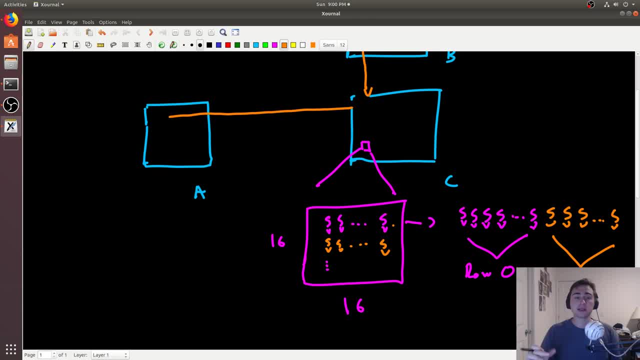 warp is going to be two of these rows of the thread blocks mixed together. So what's wrong with this? Well, now, every single time, we want to execute an instruction. So if we want to do, you know, read, or we want to do a write or something from this, A matrix here, right, they're going to be accessing two completely different rows, right? And that's a real problem, because that means we need two memory requests before all these 32 threads can even begin execution, right? So how do we fix this? Well, there's a pretty easy way to do that. So we're going to do a 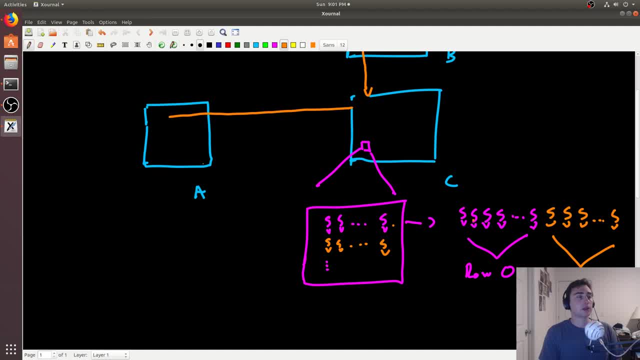 pretty easy way. What if we just increase the thread block size, right? So we just make it say 32 by 32 now. So now all of these purple threads, right, we'll have all the way here. now these will be 32 threads, right, So entire warp will be made of the exact same row of you know, in this case the A matrix, right, which is really good for us, because that means they'll be accessing one big consecutive chunk of memory. 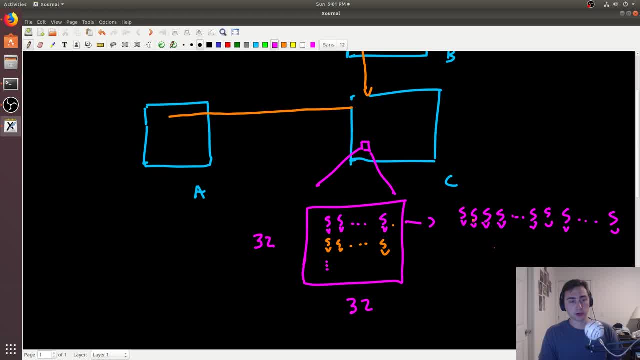 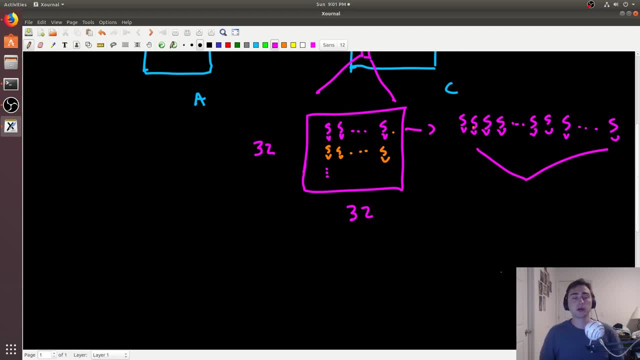 And if you're unfamiliar with how the GP memory system works, all of these threads, you know, you would think maybe you know, if you're unfamiliar with GP architecture, okay, 32 threads all accessing part of a 32 transactions, right, But there's this, there's this thing called a coalescer, right, And what that does is it'll say, okay, all these 32 threads are trying to access the exact same, or you know, a consecutive, chunk of memory. Well, instead of doing 32 requests, 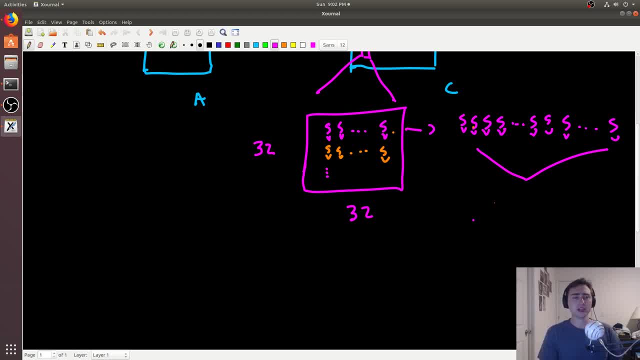 I can do one big request, right? So this will say: lead to one request from memory, right, And it will load in a 128 byte cache line. So the L1 cache works on 128 byte cache lines And that's for a very specific reason. So typically we're using things like ints or floats. floats are four bytes, ints are four bytes If we translate that to 32 threads, which is our SIMD width. if each 32 threads loads in four elements or four bytes, right, or requires four bytes, 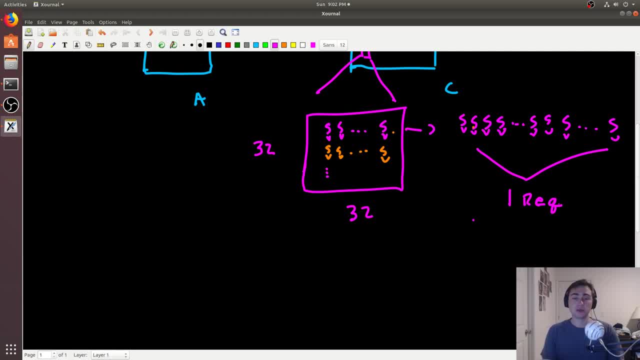 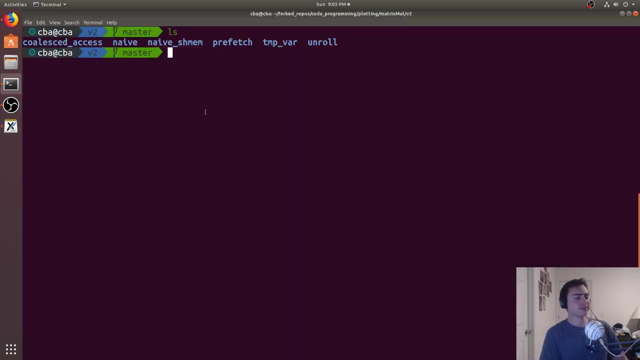 32 times four is 128,, right? So you know, one cache line fits all the ints or all the floats for a particular warp, right? So if we just change the size all of a sudden, we guarantee that we can get this one request instead of two requests, And so that will be. that's what we have here, Right? So if we go ahead and go to coalesce accesses, all we've done is we've changed one line of code again, Right? So now we've got, you know, instead of our thread block size being 16 by 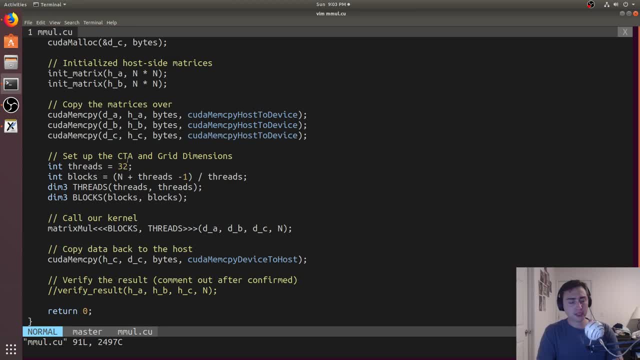 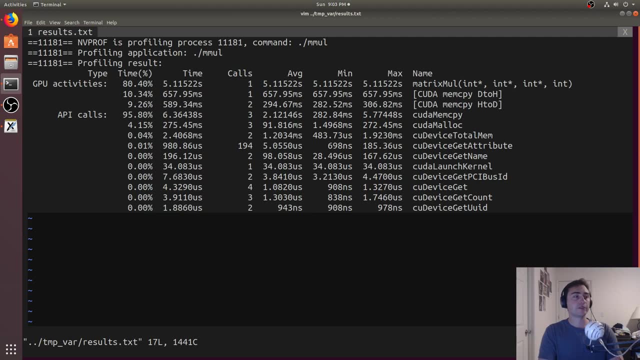 16, it's now 32 by 32.. Right, so just a single number change And it's just refresher. If we go back we go to temp var results. So we were at 5.1 seconds here, down from 13 seconds, And so once we start doing coalesce accesses, we see we're down to 4.25.. So we've improved performance by about 0.75 seconds, right. So again, you know pretty good, right Almost we have almost about an entire second. 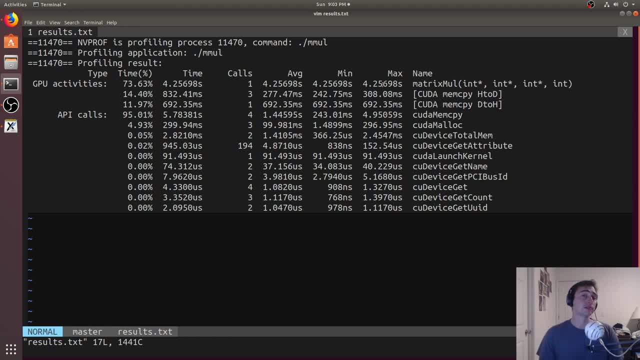 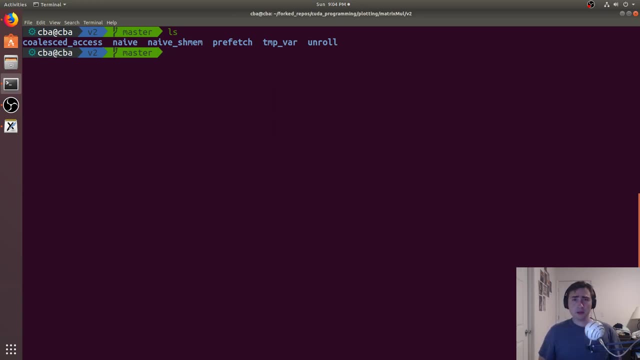 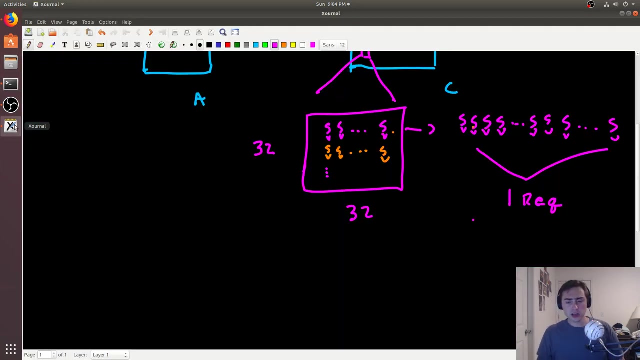 of improvement just by changing a single number, right in understanding how the hardware works. But of course, we can do better, right? So how do we do better? So let's go ahead and get exit out there. we'll go back, So the next thing we can think about. you know, even without using shared memory, we can still do some prefetching, right? So what are we going to take advantage of? So let's go back to our picture. So what we're going to go ahead and take advantage of is this idea that you know. let's go ahead and zoom. 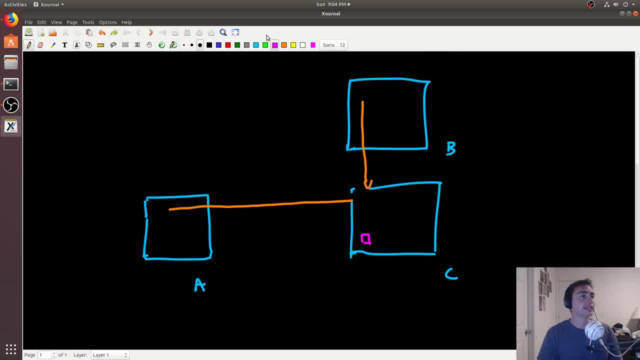 back, get rid of these. we're going to take advantage of the fact that, inside of the A matrix, for all the threads that are mapped to the top row of the C matrix at any given moment, all these threads will be accessing one element of A, but they'll be mapped to the different columns of B, right, Well, okay, so if all 32 threads inside of the A matrix are going to load in, you know? 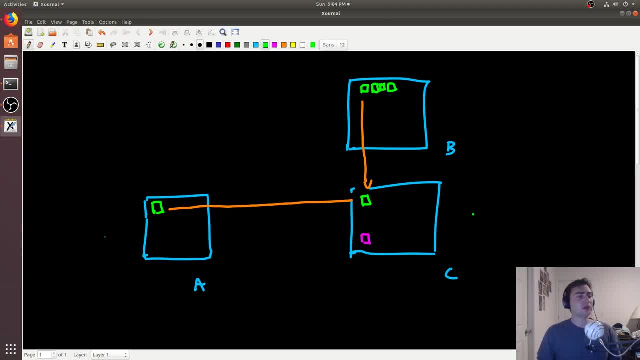 32 different columns of B but only one element of A. why don't we load in a couple of the elements of A ahead of time, right? So we'll already be kind of using up. you know all of our, you know parallelism here, So let's try to use some more inside of A. So instead of loading one element from A for every 32 elements of B, why don't we load in four elements of A? So this is kind of a form of loop unrolling. So let's go back to our code. 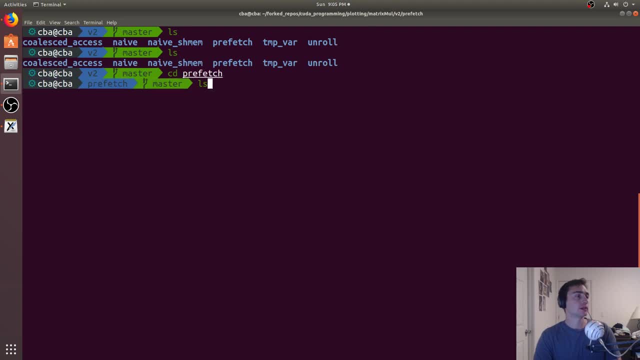 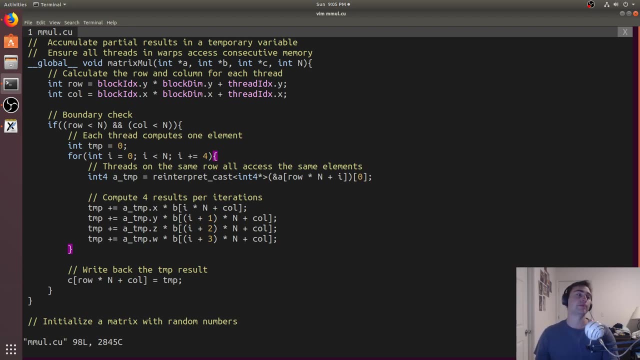 We'll go to prefetch And we'll see how we do that Right. So if we understand some of the more modern features of the language, say vectorized memory accesses, we can go ahead and load an int four. all an int four is is four integers. right, It's a struct with four fields: x, y, z and w. But what this does is it generates a wide vectorized load. So instead of loading 32 bits, right, say, for a single int or a single 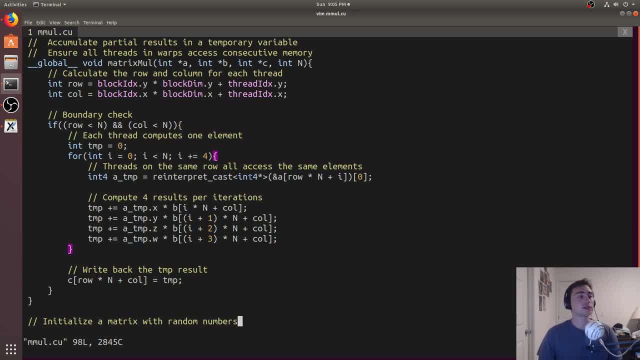 64 bits, maybe like a load64 for two integers. this guarantees that we can get a 128-bit load, so a LD64.. So in this case we'll load in four elements from A and we'll just play some tricks with casting here. 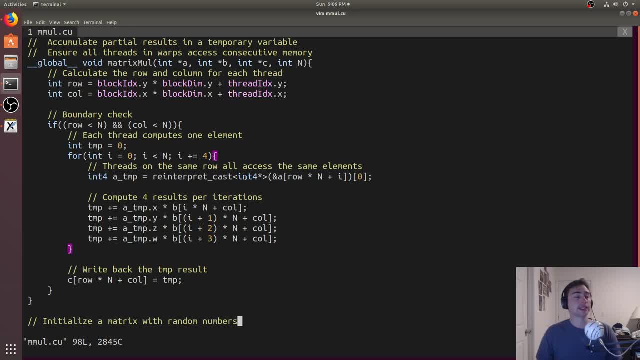 So we'll pretend that our big array of integers is actually an array of int4s, and so we'll load in one of these int4s, and that way we kind of shrunk our loop. so now it increments by four every single time. 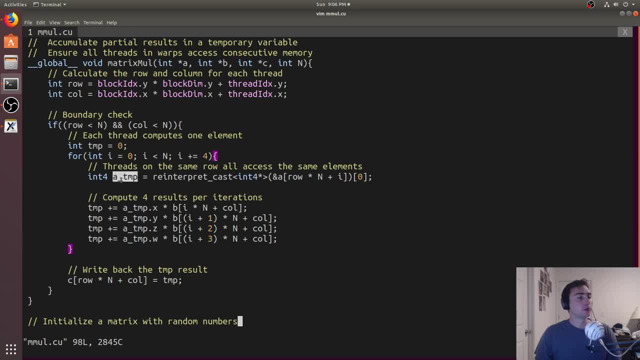 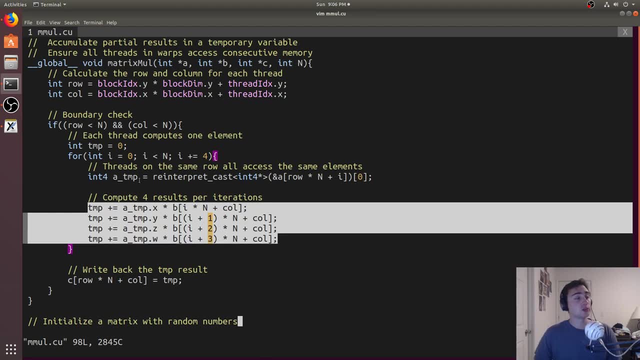 so we basically unrolled the loop by four. So we'll load in four elements, we'll put them in atemp and then here's our four computations. So instead of having four different iterations of the loop, we're now going to access x, y, z and w. 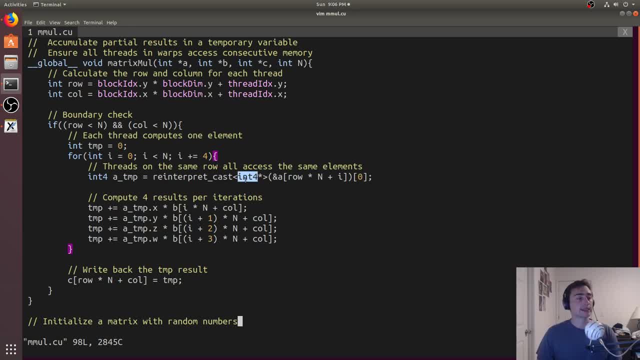 and these are coming from a single memory access. that's this wide memory access right here. And then b stays the same. we just have to increment i every single time, like it would normally be, So 0,, 1,, 2,, 3, because it gets shifted over by four every single time. 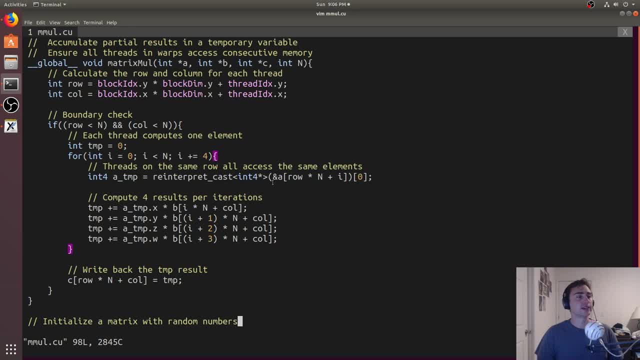 Okay, so a little bit more complicated than the last couple of optimizations, but nothing really too fancy here. All we're doing is we're saying, okay, well, when I'm accessing the b matrix, right for every single warp, it's going to be loading in 32 elements from the b matrix. 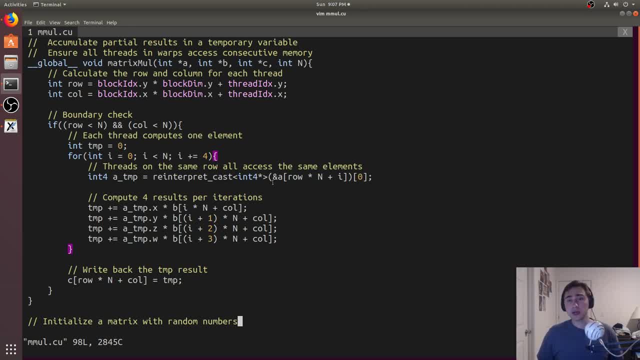 but it's only accessing one element from the a matrix. Well, I've got wide hardware. why don't I start loading in extra elements from the a matrix ahead of time, especially if I can do them in a single access, which is what we do here with this int4.. 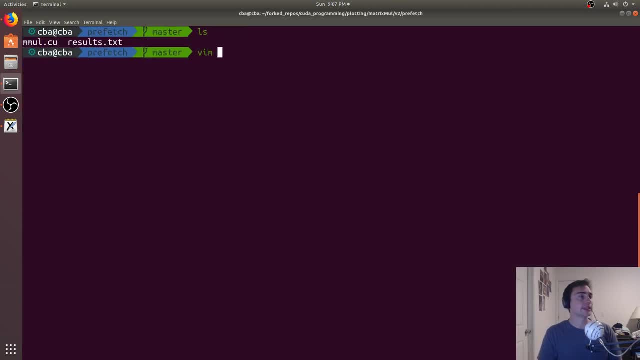 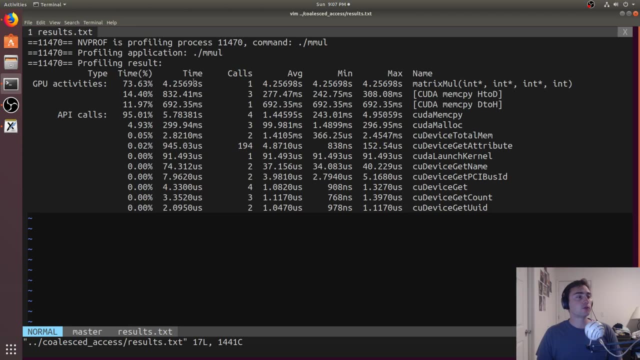 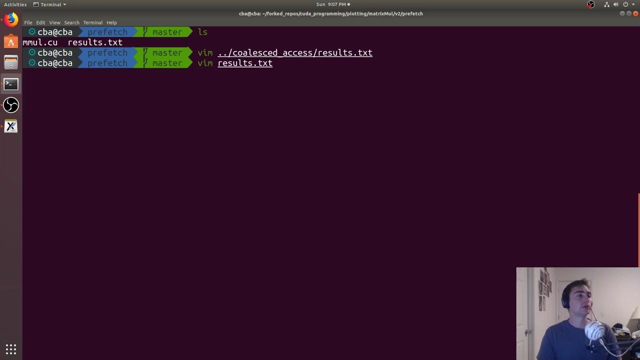 So what does this do for us? So again, let's see what we did with the last optimization. So we did coalesced accesses resultstxt. we got 4.25, about 4.26 seconds, right. And so now we went from 4.26 to 3.5, right. 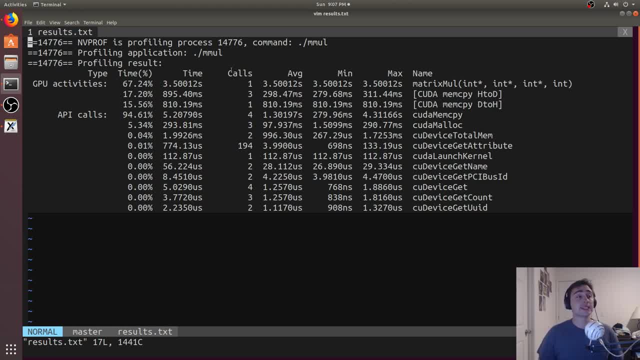 So again about 0.75 seconds. so about three quarters of a second decrease just from doing a little bit of prefetching here and making sure that we're using the hardware effectively. We know we can do, you know, vectorized loads in some circumstances. 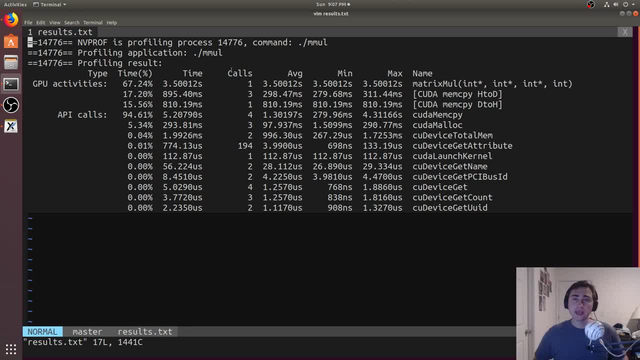 Maybe the compiler isn't smart enough to figure that out for us. So if we can help the compiler along, well, we just gained another. you know, three quarters of a second, you know, basically, but not too much effort, But of course we can still do better, right. 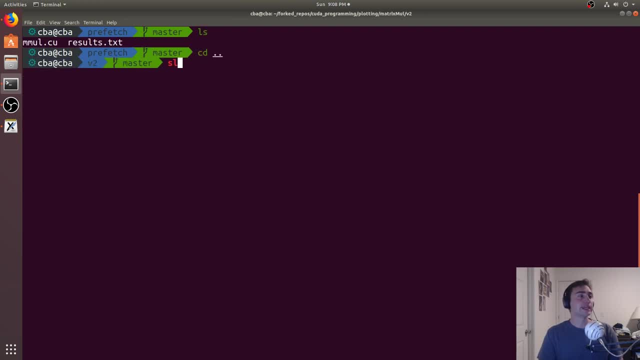 So now, what have we done? Let's kind of recap a couple of things. One: we went from a baseline version. The next thing we did was we accumulated a temporary variable to limit the number of accesses to memory we have or unnecessary accesses. 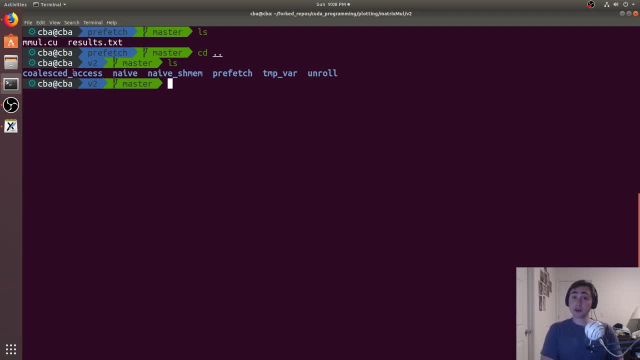 Then we saw that we could get better coalescing if we just made sure that all of our threads in each warp were on the same cache line. Then we saw that, you know, if we went ahead and prefetched some elements ahead of time and use these wide vectorized loads, 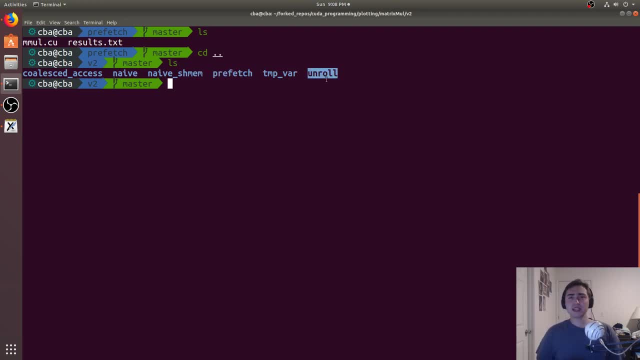 we could get even more improvement. Now let's see what we can do with some unrolling. that's not manual, right? We don't always want to do some manual unrolling. Sometimes it's necessary because the compiler isn't smart enough to unroll the loop properly. but it turns out sometimes it's okay. 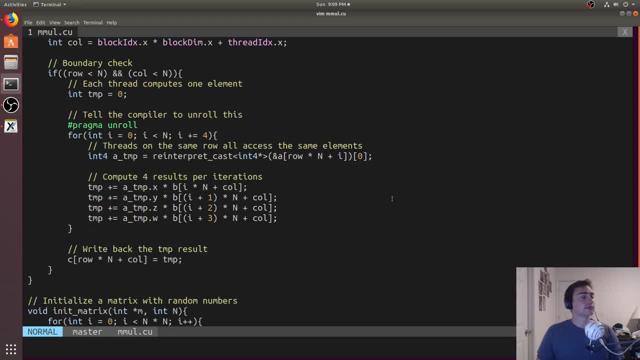 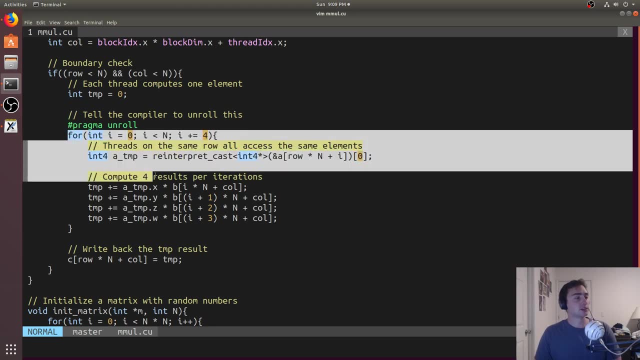 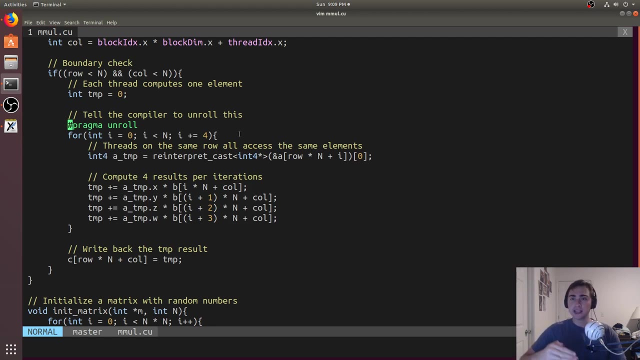 So we can add just a single line for some circumstances. So we can add this pragmaunroll and it will attempt to fully unroll this loop right? So if you're unfamiliar with loop unrolling, instead of having a loop it just basically puts all of the iterations of the loop, one after each other. 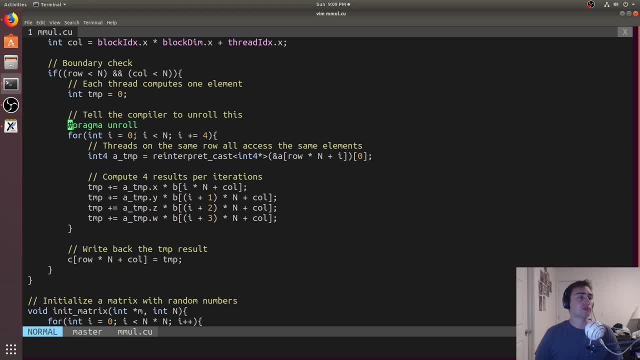 right inside of the actual assembly, right, And it gets rid of some of the loop overhead of, say, doing conditional checks, incrementing loop counters. you just have all the code there, So your code gets bigger, but you get rid of some of these checks, right. 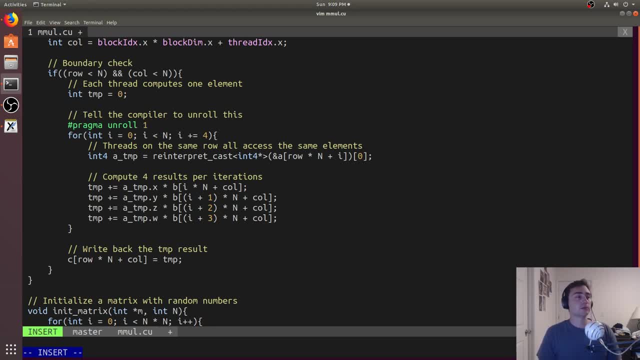 And you can even specify this So you can say: unroll one right, which basically just means: don't unroll the loop. You can unroll it twice, four times, et cetera, or you can try to fully unroll the loop. 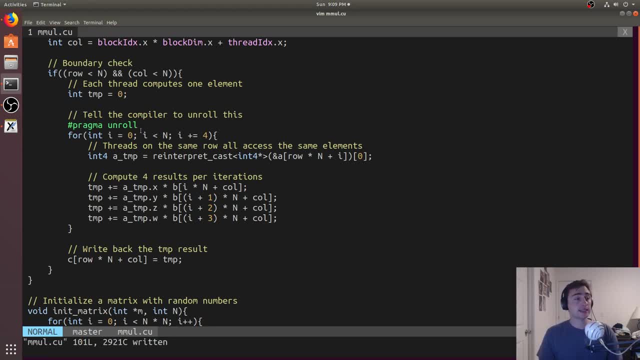 So nothing else. Nothing else has changed, right? So the grid size stays the exact same, the thread block size, all this prefetching stays the exact same. All we're doing is we tell the compiler with this pragma: hey, unroll this loop. 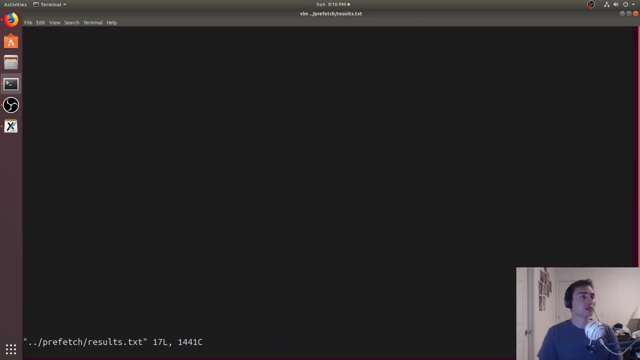 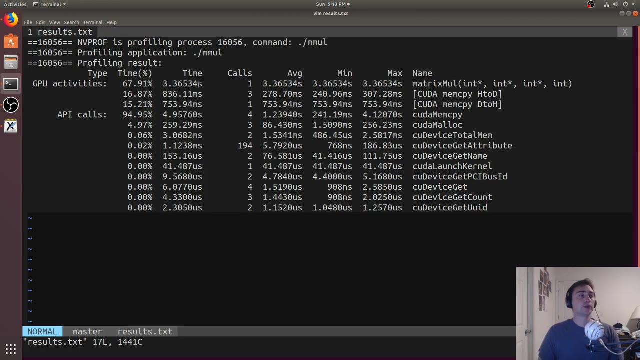 So again, we'll go back to the prefetch and we'll look at the results. We were at about 3.5 seconds right And here right, we're down to about 3.36 seconds right. So it's not a huge improvement, but again, it's a single line of code. 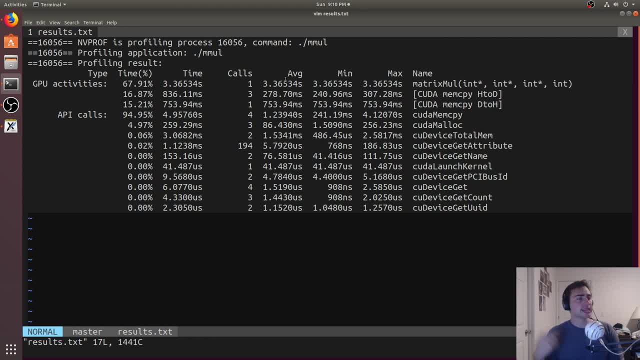 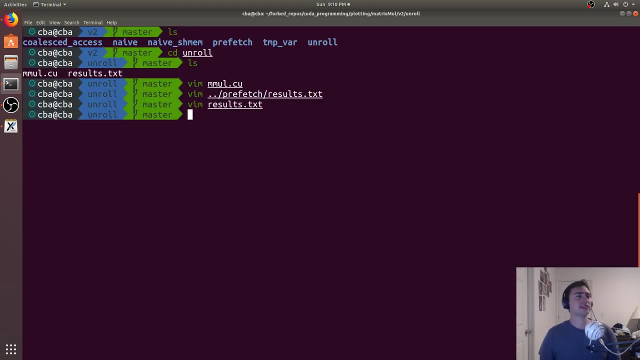 And it is stable around this. So this isn't just an individual run thing. I tested across a couple of runs. It'll vary slightly between each run, but about 150 millisecond improvement for that single pragma. Now a lot of this is kind of like: OK, well, 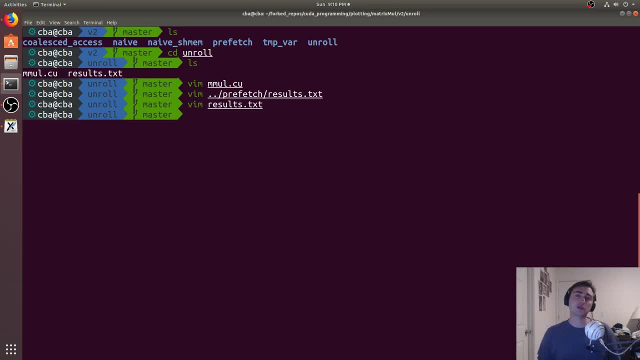 why are we trying so hard to improve matrix multiplication without using shared memory? And the real key point behind this is: what's actually better? Is it better to spin all this time Doing all these crazy optimizations- or maybe not so crazy optimizations- without using shared memory? 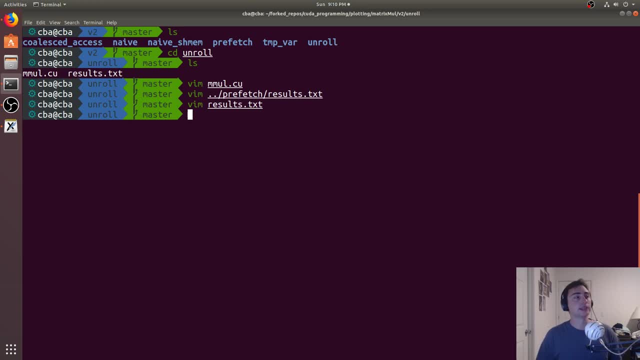 Or should I just use shared memory? And the real kind of lesson to be learned here is that it's just really important to understand the hardware. So let's go to a naive oh, go back a directory. So let's go to a naive shared memory implementation, right? 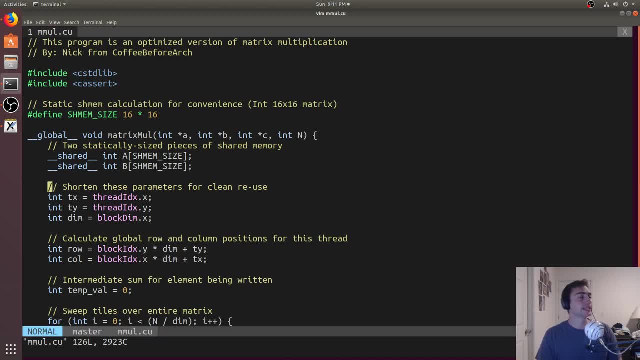 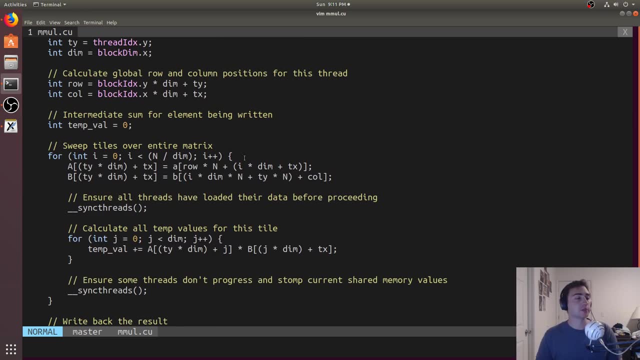 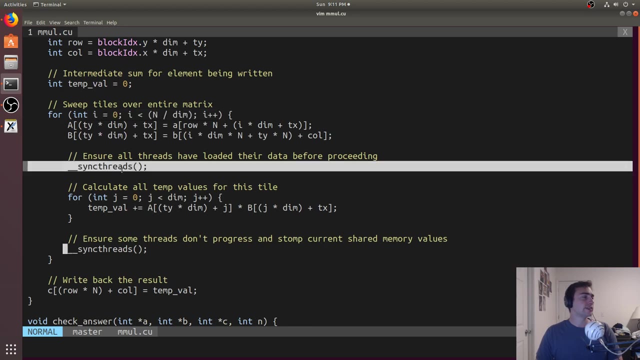 So here- this was from another example that I did in the CUDA crash course series, And it basically just does basic matrix multiplication using shared memory. It uses 16 by 16 thread blocks And here you see, it just iterates the tile over loads in the values. 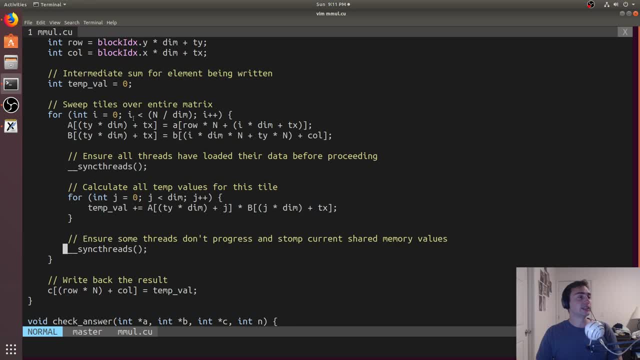 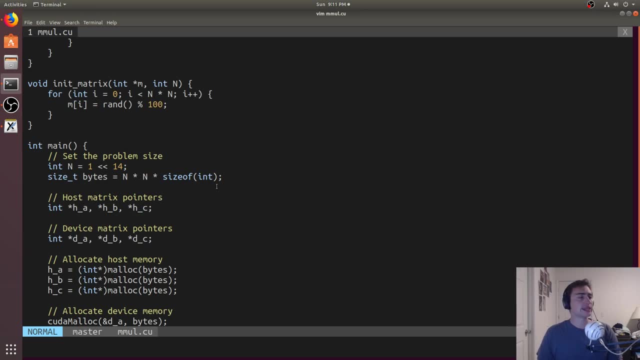 and then computes on the individual tiles before loading in a new tile right And again, like I said, it uses 16 by 16 thread blocks, which we already showed is not ideal, right, We can do better if we maybe make them 32 by 32.. 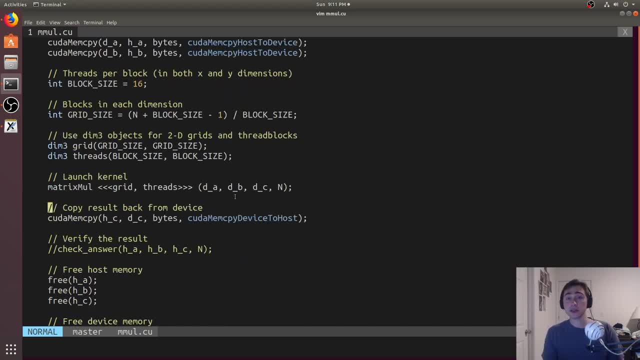 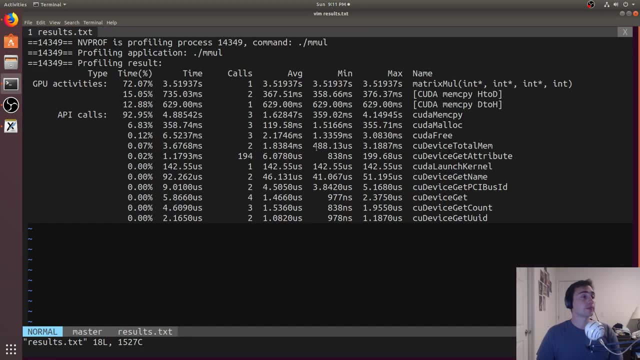 So let's see what happens if we just throw shared memory at it, without considering, maybe, any of these other details. So I've got the results here for a 2 to the 14 by 2 to the 14 matrix And it's about 3.5 seconds right. 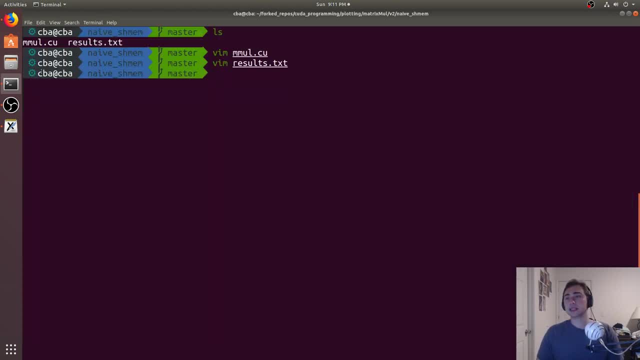 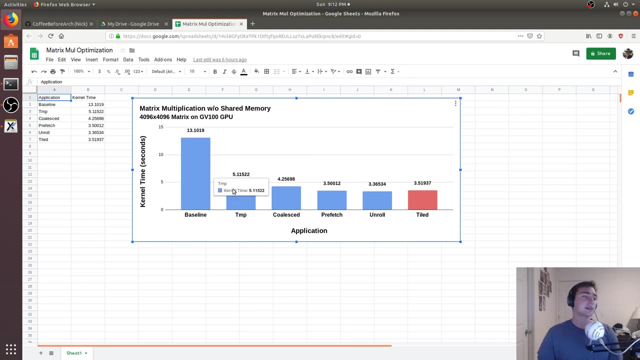 So, to put this in perspective, I went ahead and plotted these out, these different optimization stages, and I've got them right here. So here's our baseline at about 13 seconds. We get it down to about 5.1 seconds by adding a temporary variable. 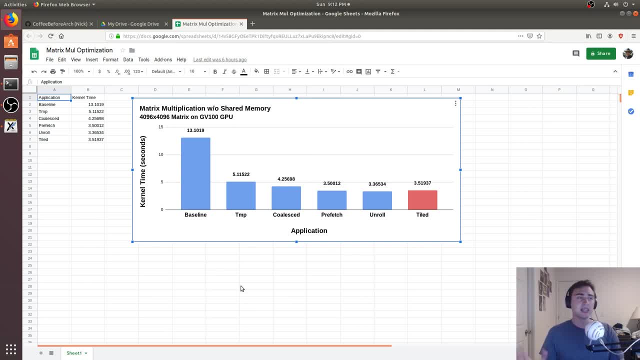 coalescing from 5.1 to 4.25.. So a little less than a second here, maybe about 0.85 seconds, another 0.75 seconds by doing some prefetching, another 0.1, 0.15 seconds or so 0.16 seconds from doing this loop unrolling. 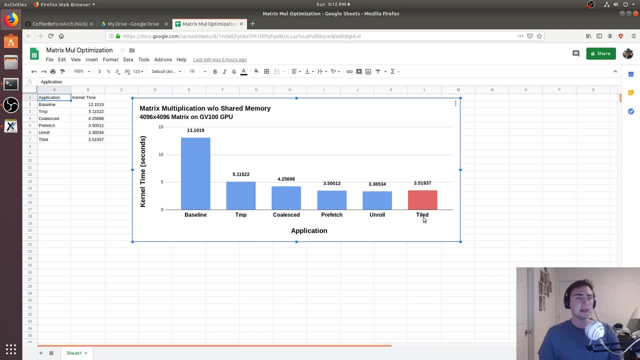 And we see that that kind of naive tiled approach it's at 3.5 seconds, right. So that's worse than even just the prefetch version, right. So the key point here is just it's really important to understand your hardware and understand. 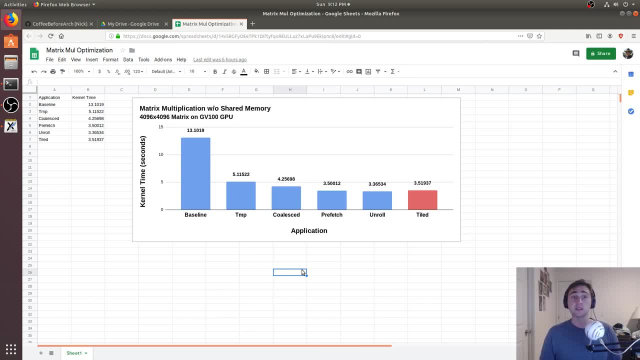 why you're writing the code that you are and how that's going to translate to performance. So, on different machines, like I said, you know you may not see quite as drastic speed ups. You know even a different matrix size. you'll see a different speed up potentially. 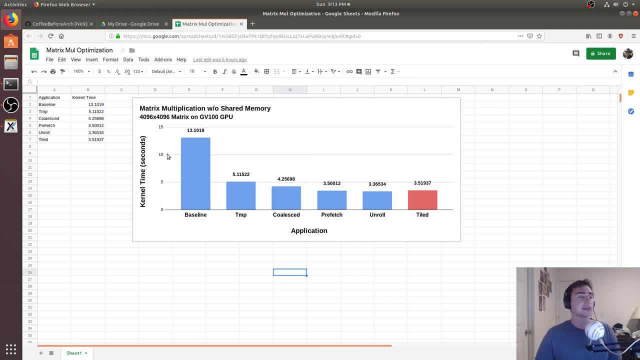 But the important thing is understanding why that speed up is occurring. right? So between the baseline and the temp we're just having less writes to memory. right So we're just having a single write at the end of execution, And when we have a ton of threads, that's way less writes or way fewer writes. 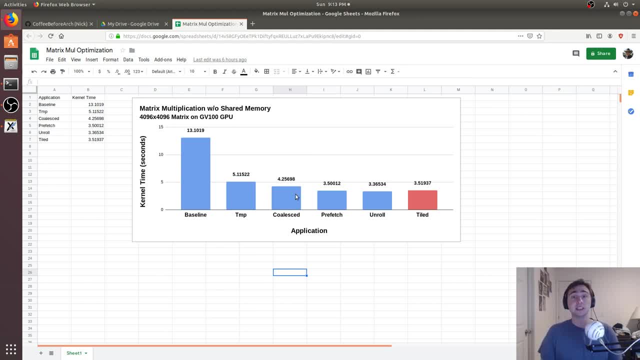 When we're coalescing, we're making sure that you know again we're not generating excess. you know reads from memory. We just need to read you know one time for each warp. Now, with prefetching, we're making better use of our hardware by doing these wide vectorized loads right. 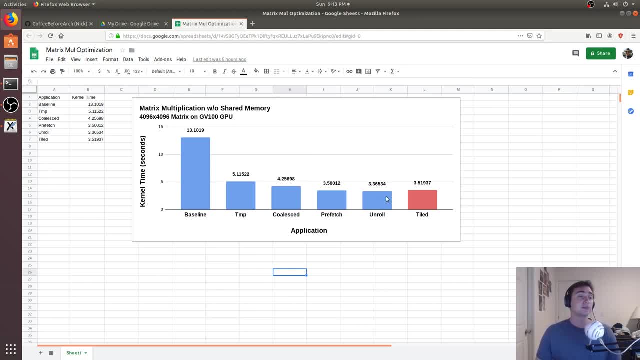 And then we have these values available to us ahead of time, And then, with loop unrolling, we're getting rid of some extra loop overhead, just by understanding what the compiler can do right. And this is without using, you know, cache tiling at all.